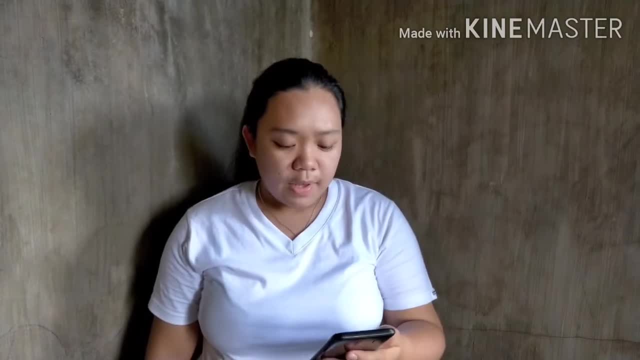 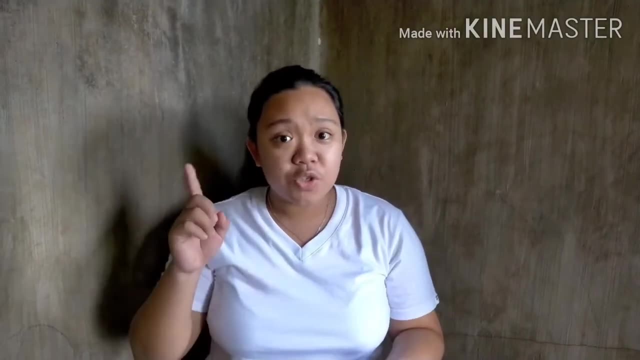 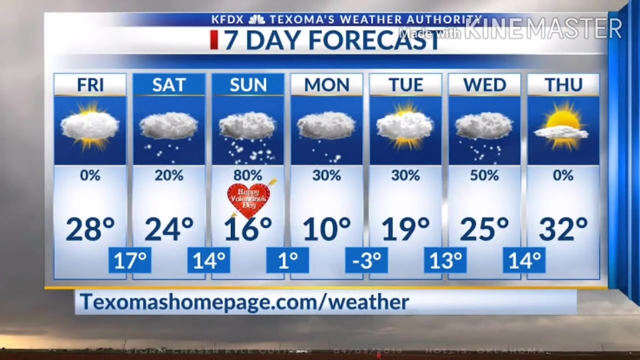 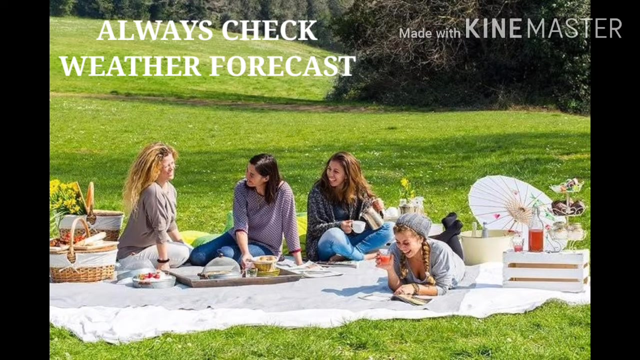 Probability has something to do with a chance. It is a study of things that might happen or might not. We use it most of the time and usually without thinking of it. There are numerous applications of probability in real life: The weather forecasting: Before planning for an outing or a picnic, we always check the weather forecast. Suppose it says that there are 70% chance that rain may occur. 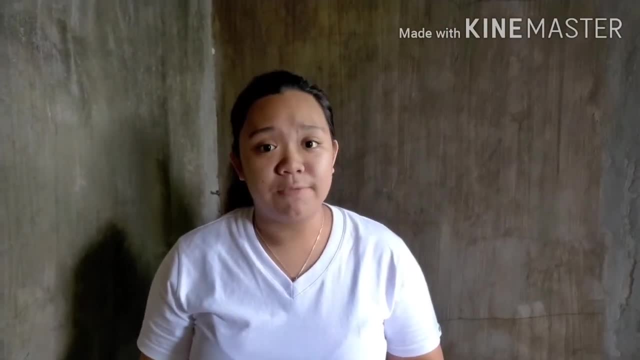 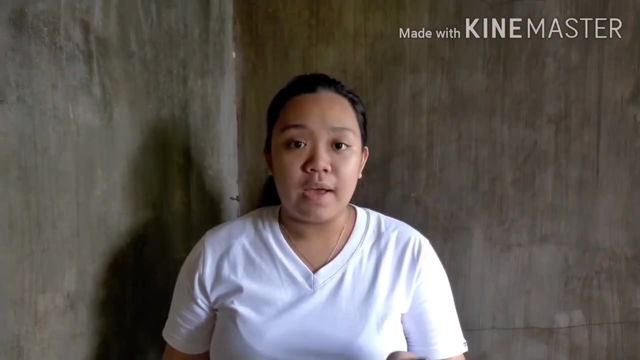 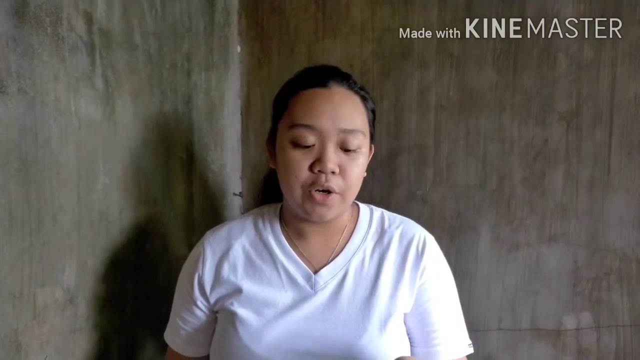 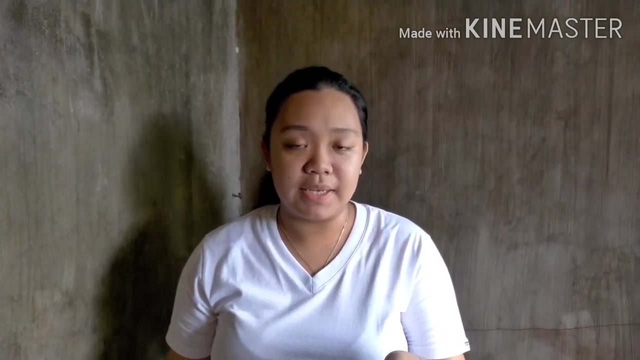 Do you ever wonder from where these 70% come from? Meteorologists use a specific tool and technique to predict the weather forecast. They look at the all other historical database of the days which have similar characteristics of temperature, humidity and pressure and determine that on 70 out of 100 similar days in the past it had rain. 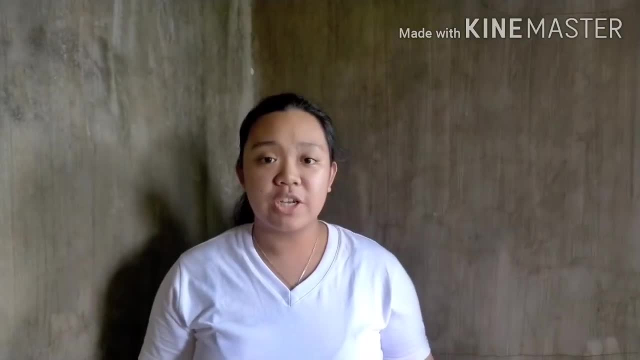 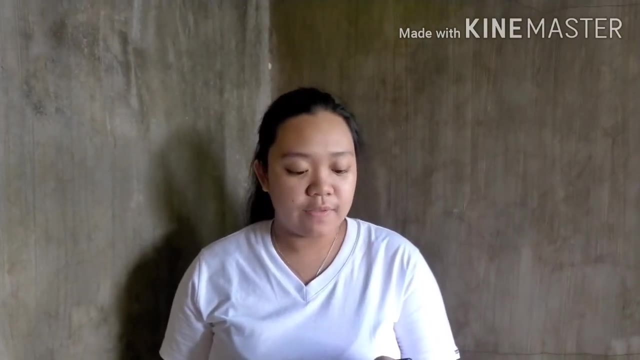 In medical decisions. When a patient is advised to undergo surgery, they often want to know the success rate of the procedure. They often want to know the success rate of the procedure. They often want to know the success rate of the procedure, Which is nothing but a probability rate. 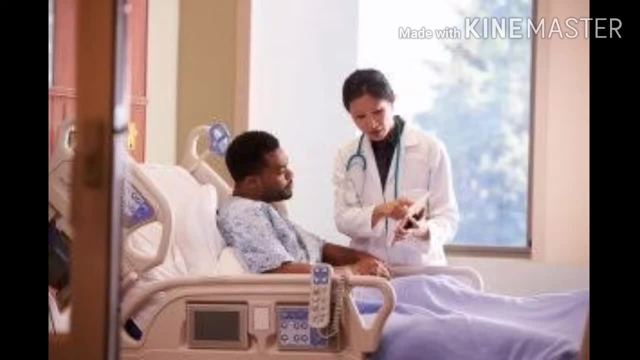 Which is nothing but a probability rate. Based on the same patient. takes a decision whether or not to go ahead with the same. Based on the same patient takes a decision whether or not to go ahead with the same. Based on the same patient takes a decision whether or not to go ahead with the same. 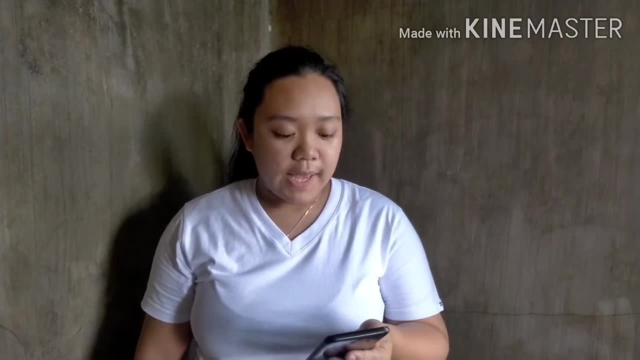 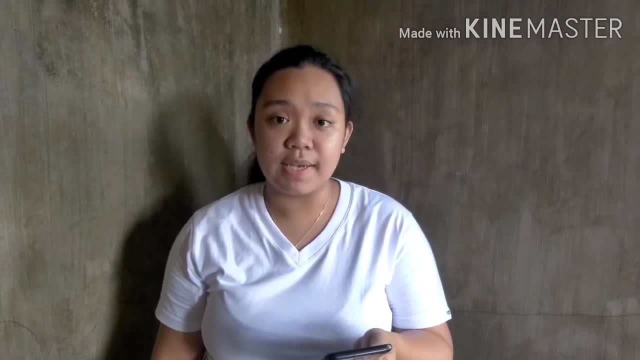 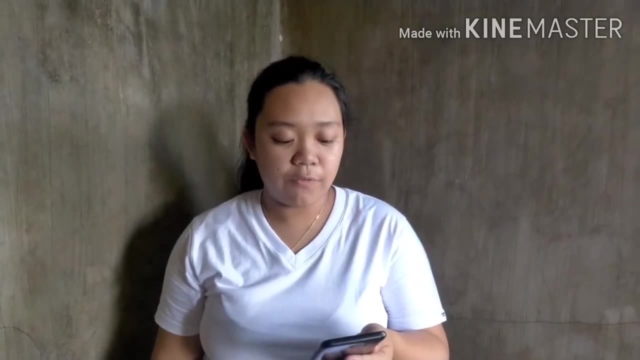 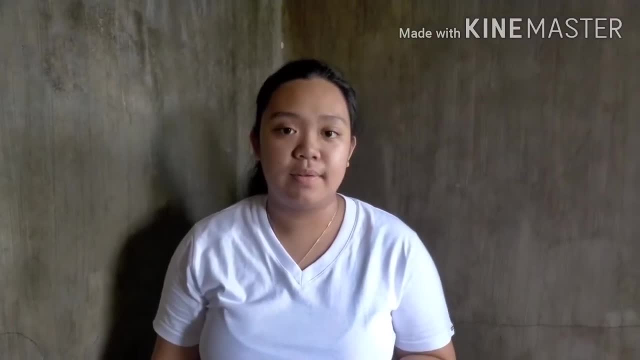 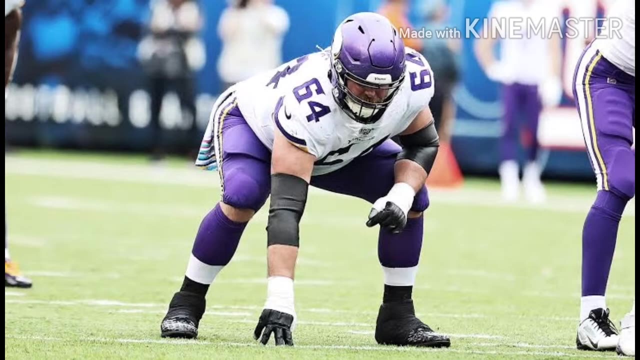 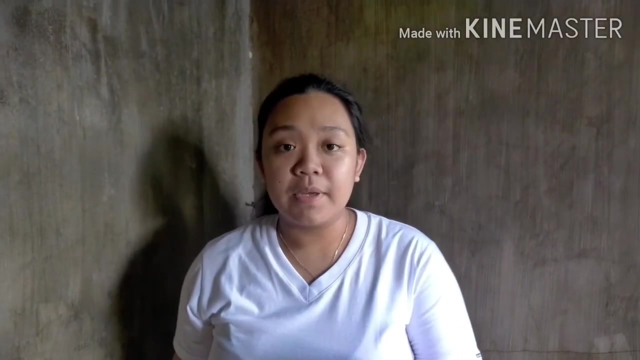 regarding the team's performance and members in the sport. Example of this is the probability of how many tackles a defensive lineman makes in American football. In politics, many politics analysts use the tactics of probability to predict the outcome of the election's results. For example, they may predict a 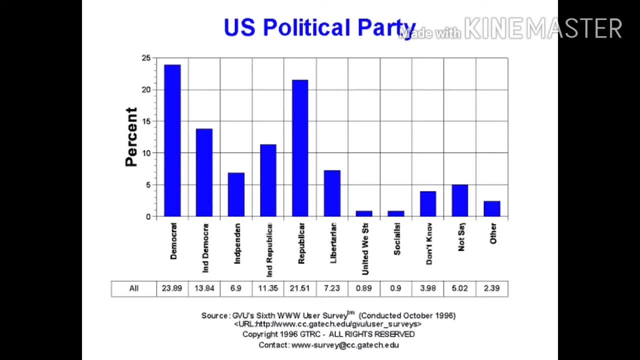 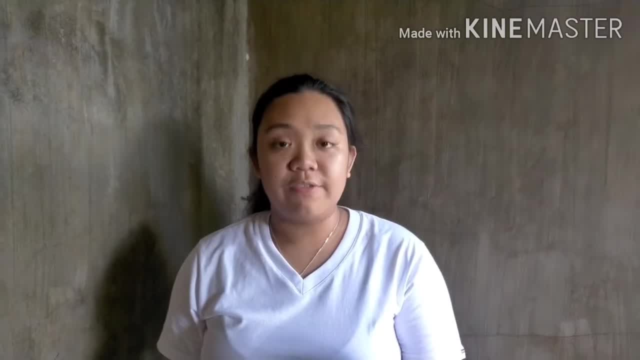 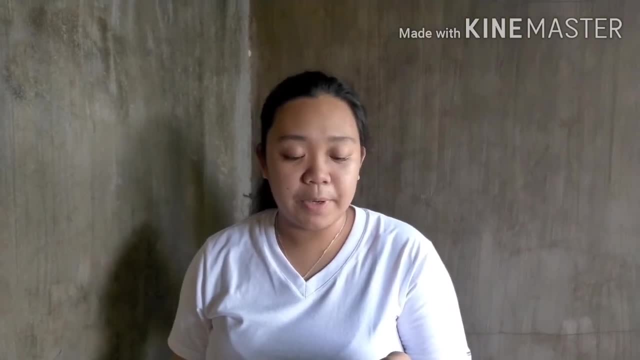 certain political party to come into power based on the results of exit polls. Insurance Insurance companies use the theory of probability or theoretical probability for framing a policy of completing at a premium rate. The theory of probability is a statistical method used to predict the possibility of